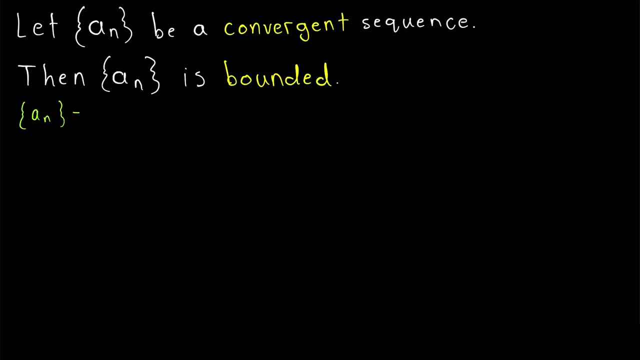 some sequence- a, n- that converges to a number, let's say a. Then by definition of a convergent sequence we could pick any positive number, epsilon that we want, Let's say epsilon equals one, and it would follow by definition. there exists some natural number, big n, so that for all terms of 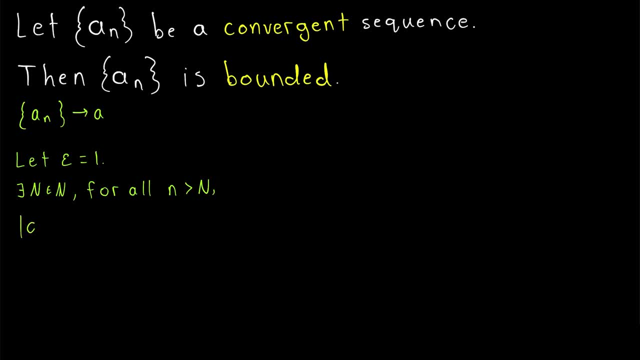 the sequence. after the big nth term we have that those terms of the sequence are within one of that limit a. So the absolute value of a, n minus the limit a, is less than one. Again, this is just by definition of the sequence. 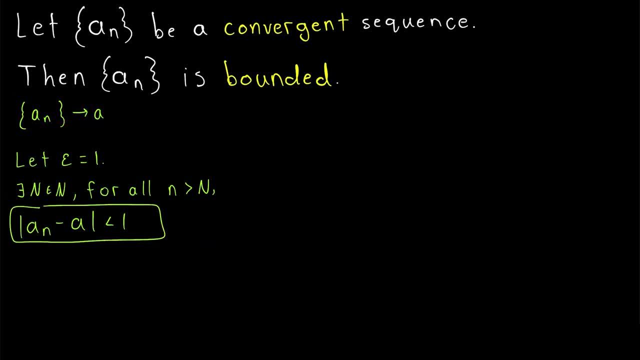 a n converging to a. this absolute value inequality is equivalent to writing that negative one is less than a n minus a without the absolute value bars which is less than positive one. I'll leave a link in the description to my lesson proving that this is equivalent to this. it is a very important. 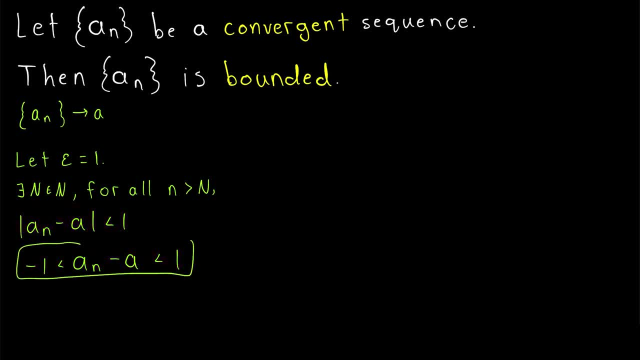 result. we use it a lot. Then the big idea is we can add a through this inequality to have that a minus a. So a minus one is less than a, n is less than one plus a. In other words, we have a lower bound, a minus one, and an upper bound, one plus a, for all terms of the sequence. after the big nth term, we've guaranteed that all terms of the sequence after a certain point are bounded between a minus one and one plus a. there is only a finite number of terms left in the sequence to account for, So we should be able to do this. 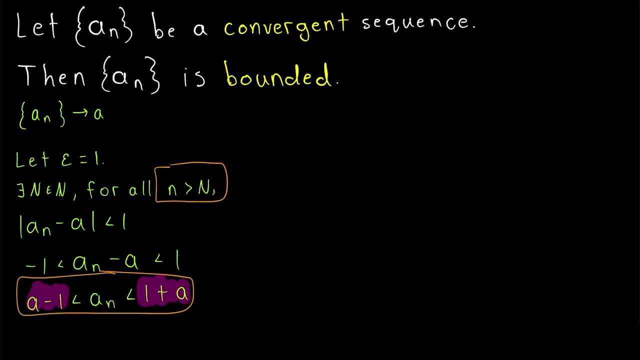 So we should be able to adjust our argument to make sure that it works for all terms of the sequence. Let's see how we can finish things up. We might start with a tentative upper bound u of one plus a. We know that this is an upper bound for all terms of the sequence after the big nth term. Similarly, we might start with a tentative lower bound of a minus one for similar reasons And again by definition of a convergent sequence, we are sure that these bounds work for a minus one. 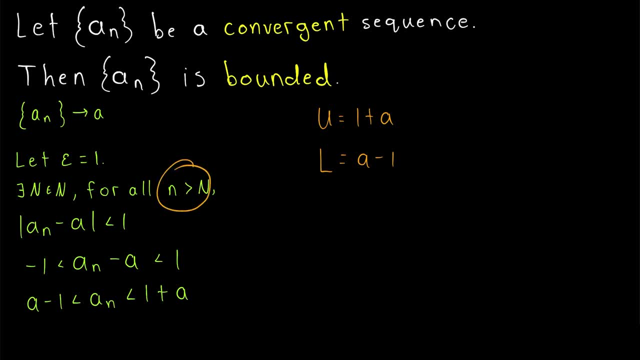 every term of the sequence after the big nth term. So the only terms left that we haven't accounted for are the first big N terms of the sequence: a one, a two and so on. through a big N, it's possible that one of these numbers is actually bigger than one plus a, in which 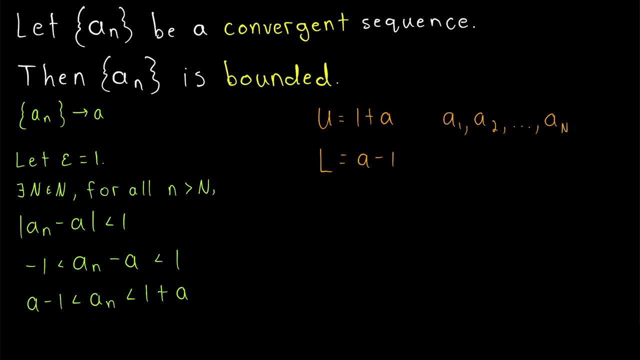 case, we could increase our upper bound u accordingly. In order to actually do that, we'll use the maximum function. So an upper bound of one plus a might work, but just to guarantee that our upper bound will work for all terms of the sequence, since that's what we actually 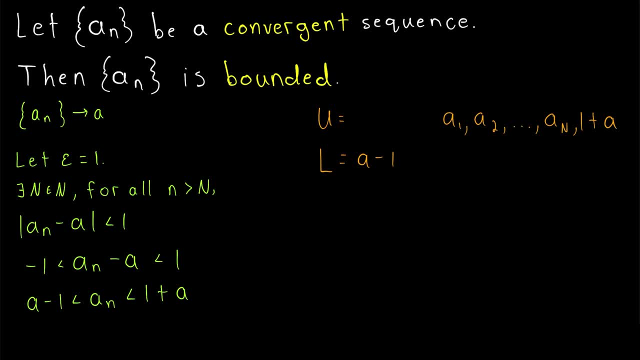 need to show, to show that the sequence is bounded. we'll let our upper bound u be the maximum of all of these numbers, And similarly for l. it might be the case that one of these numbers is less than a minus one, in which case we could decrease l accordingly to make: 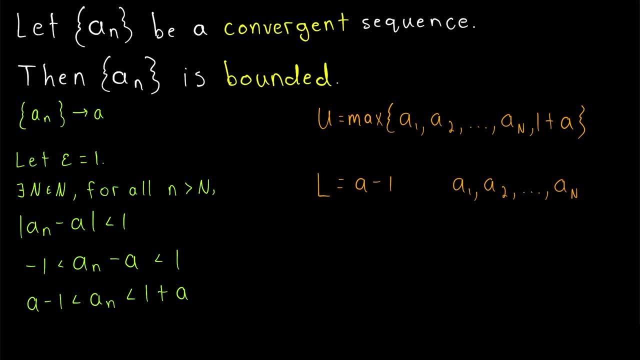 sure that we still have a maximum of one plus a. So that's what we're going to do here. So we'll let l be the minimum of all of these numbers, And that's it. u is an upper bound on the sequence, it's greater than or equal to every term of the sequence And l is a lower bound on. 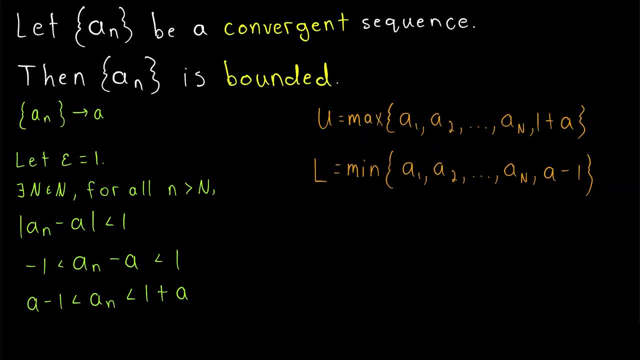 the sequence, it's less than or equal to every term of the sequence. So we have that l is less than or equal to a n and a n is less than or equal to u for every term of the sequence, a, n. And let's just recap how we. 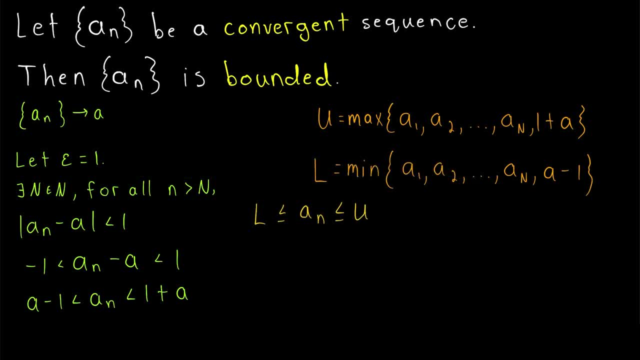 know, this inequality holds for every term of our sequence when n is less than or equal to big n. So we're looking at the big nth term and terms that precede it. well, u is the maximum of a set that contains all of those terms. So certainly u is greater than or equal to those. Similarly, 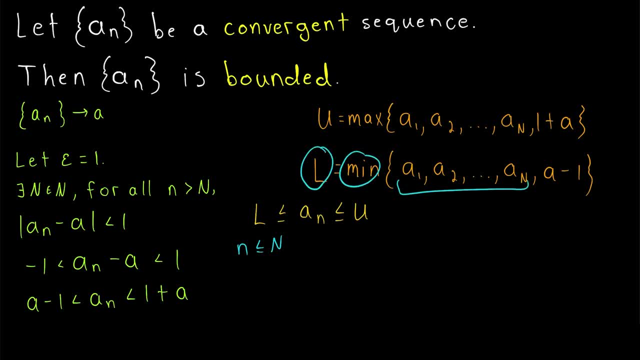 l is the minimum of a set containing all of those terms. So certainly l is less than or equal to all of those terms. Remember the only terms a, n with n, less than or equal to big n. those are accounted for in these sets: a one through a big n. On the other hand, for terms of the sequence, a- n where n is greater. 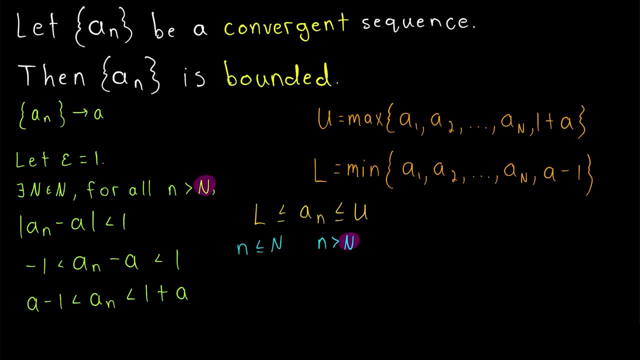 than big n. big n was selected specifically using the definition of a convergent sequence to ensure that all following terms lie between a minus one and one plus a. since one plus a is greater than or equal to big n, So we have a n less than or equal to big n, So we have a n less.